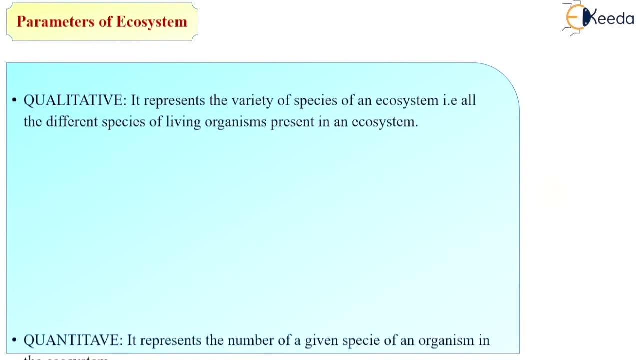 The parameters are either in form of qualitative or in form of quantitative. Qualitative form of ecosystem represents the variety of species of an ecosystem, That is, all the different species of living organisms present in an ecosystem, And quantitative ecosystem represents the number of given species of an organism in the ecosystem. 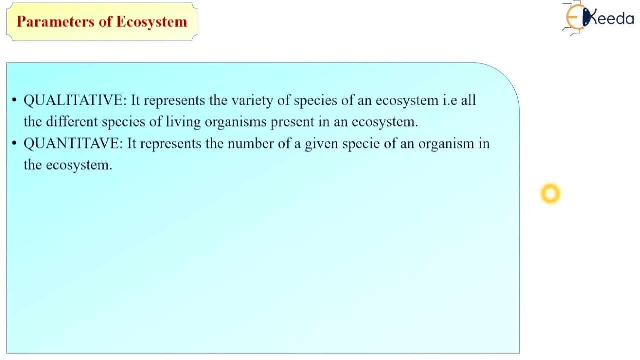 So can you differentiate these two types, that is, qualitative and quantitative? Next, a change in any of above parameters causes a dissonance In the stability of the ecosystem, which can become a variety of very important conditions of human life with time. That means, suppose, in quantitative ecosystem that means a number of given species of an organism in present in ecosystem. 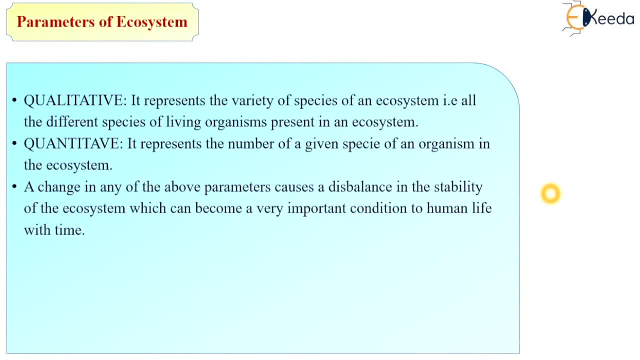 So suppose this number is reducing or will getting increased, Then that will affect to overall ecosystem, Then that will affect to overall ecosystem Or that will affect to directly to the human life with time. So it is necessary to balancing this quantitative and qualitative type of ecosystem. 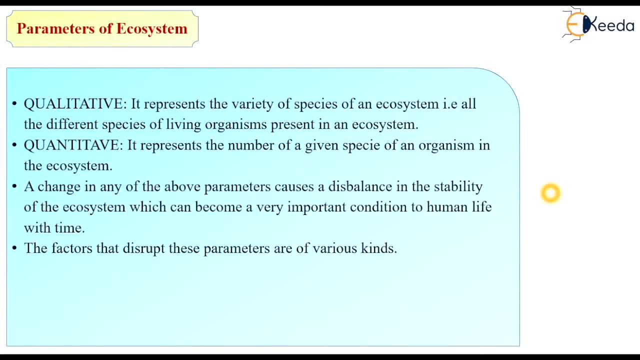 The factors that disrupt these parameters, that is, qualitative and quantitative parameters, are of various kinds. A set of ecological factors that help to provide the normal vital activity or parameters of a given kind of organism Is called as ecological nitrate. That means let's we see the overall factor affecting, or parameters on ecosystem. 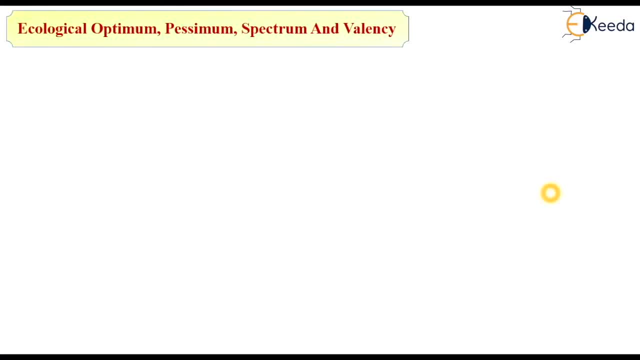 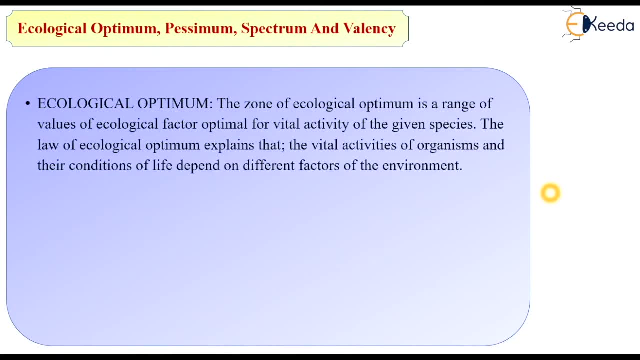 So there are again classified into ecological optimum parameter, Pessimum parameter, Spectrum and ecological valency. So let's we see one by one. parameter First is ecological optimum. That means the zone of ecological optimum is a range of values Of ecological factors optimal for a vital activity of the given species. 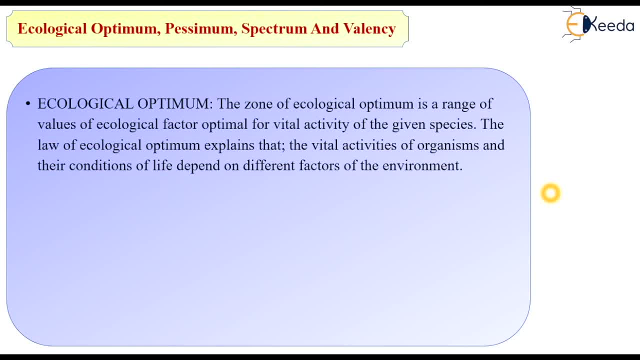 The law of ecological optimum explains that the vital activities or important activities of organisms and their conditions of life depends on the different factors of environment. That means these important species or organisms present in atmosphere, present in biosphere, Which are dependent on the factors of environment.